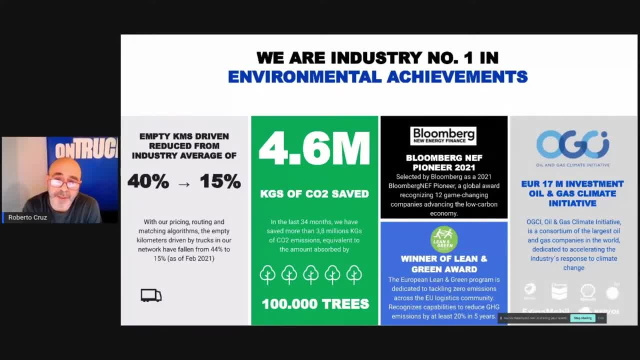 in the market and it had been observed by different companies like uh, lean and green, we. we win the the lean and green hour because we were able to demonstrate that we are reducing the co2 emission. we won the bloomberg net pioneer 2021. we were selected by bloomberg. 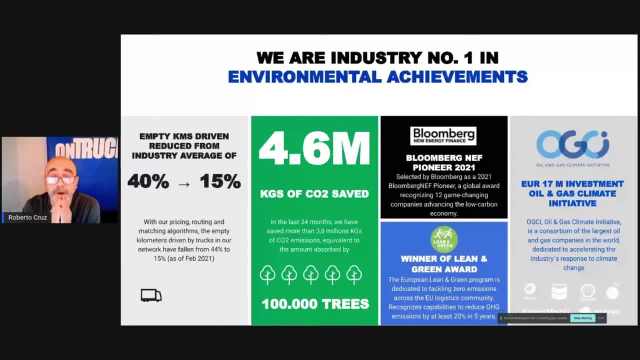 as a global recognition in a with other 12 companies. okay, uh, because, uh, they realized that we have a huge impact into co2 emission. uh, today we are uh reducing the emission to the atmosphere on four million, uh, four million dot seats. uh. a kilogram of co2, this means around 100 000 trees that have been planned. 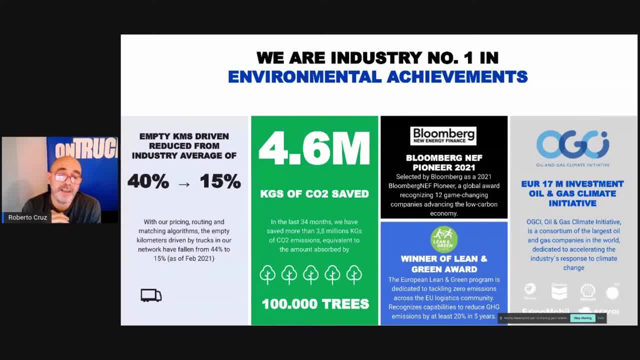 the equivalent is we plant 100 000 trees and we get an investment for oil and gas climate initiative, that is. the ogci is a consortium of the largest oil and gas companies that want to invest in companies that reduce the co2 emission, just improving the the market. 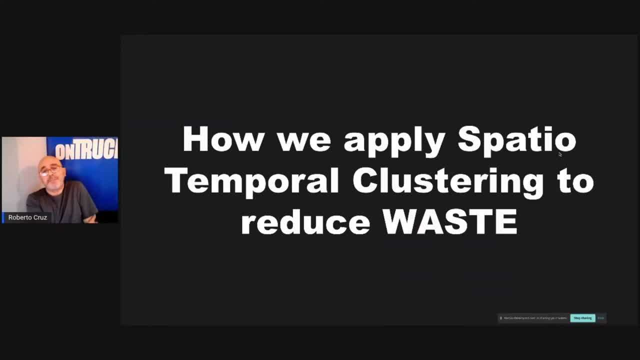 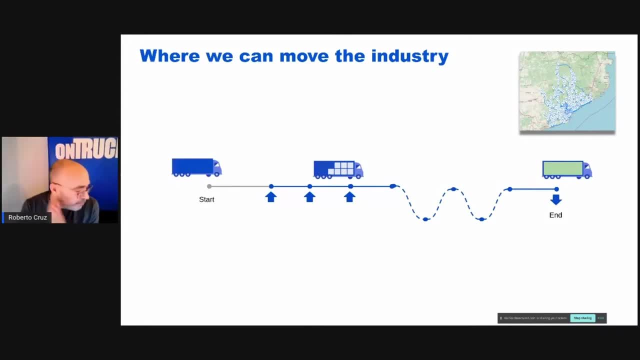 well, and then how we apply a spatial temporal cluster to reduce waste is that's the question. okay, you start moving. the industry we have, uh, our industry many times see this problem as a linear problem. this means that the uh truck start a road and starting pick up, uh, picking up. 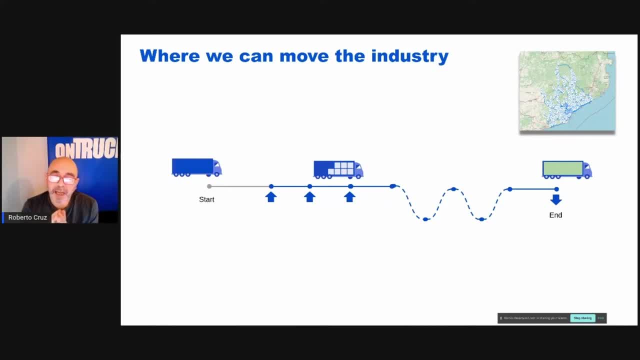 uh, loads and and full load or not full load, uh, when they have to store. normally we have several constraints. we have time windows constraint, we have our service constraint, we have a kilometer that we can write load weight- many constraints that we have to consider. normally we 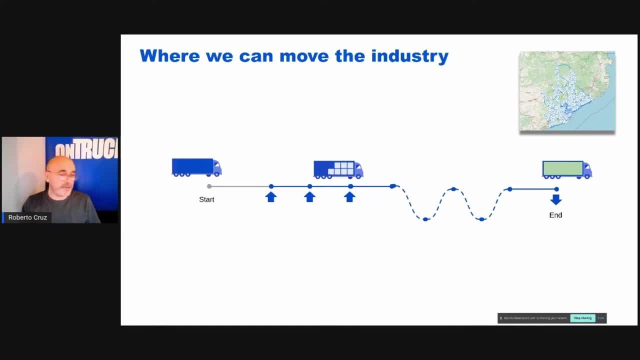 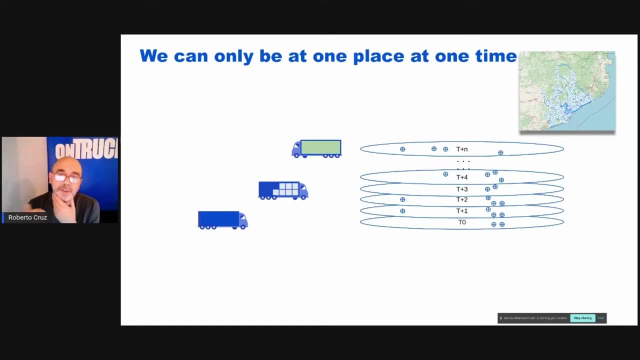 solve this with, uh, with some algorithms, uh, heuristic algorithms- But what we propose is just to use another kind of solution, because when we start, we cannot see this as a linear. We have different space of time in which we have t0, in which we have two orders that we have to collect. 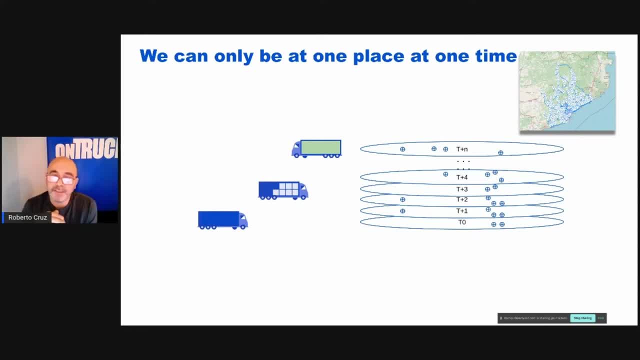 In t plus one we have four orders. We maintain this four order in t plus two, but in three plus three we have two different orders. This means that our linear view isn't changing. It's changing across the time. We have four dimensions. We have the spatial dimension in which, where we have to pick up or drop the order and the time in which those orders are available. 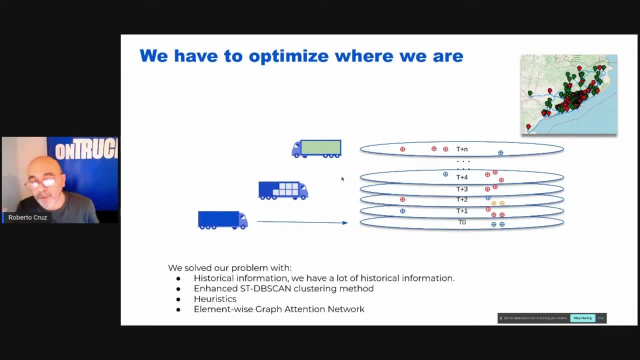 What we have to do is just select the bedroad across those this spatial and time dimension, in order to improve first, the vehicle utilization, reduce the kilometer that we drive and therefore reduce the CO2 emission per ton that we are moving. How we solve this problem? Well, we solve it with historical information, Historical information. 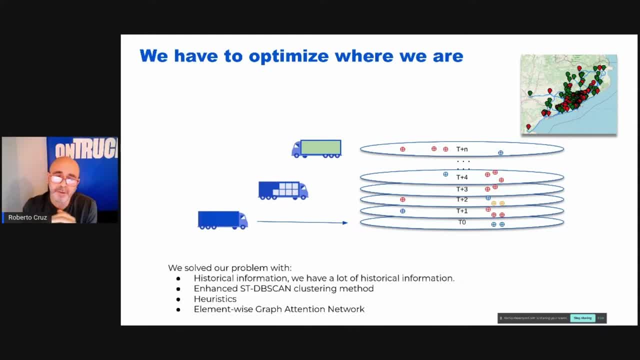 because we have a lot of historical information. With this information we can create, pre-calculate a cluster. How we pre-calculate clusters. We pre-calculate clusters with enhanced STDBSCAN clustering methods. What we call enhanced is an internal version that we developed in that based on STDBSCAN. 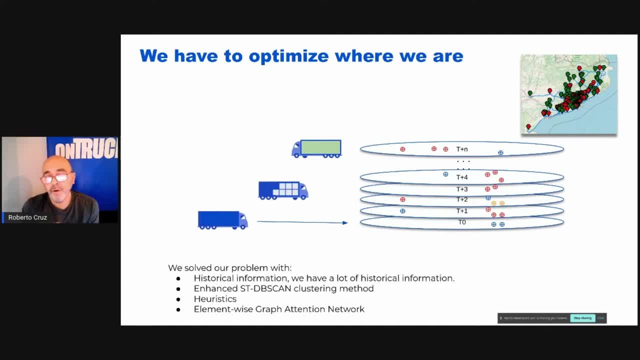 we are able to look in other moments of time and we are able to cluster sites not only across the space and time, just like a time machine. This means that we can simulate where we are in any point of time With heuristic. okay, we use heuristic to solve the routing problem. 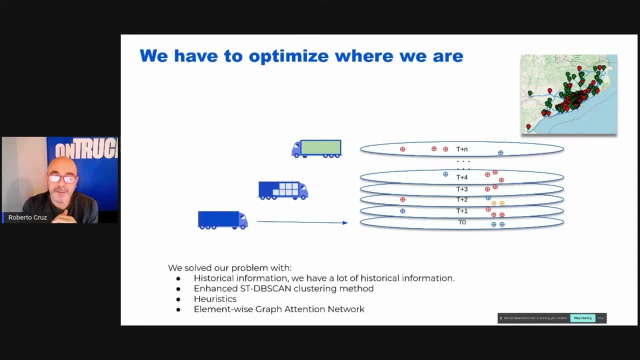 the basic, heuristic problem and with the most important part, that is, the part that is learning about the reality of the situation, that is, a neural network that is element-wise, graph attention network. This allows us to center ourselves on the edge of the network. 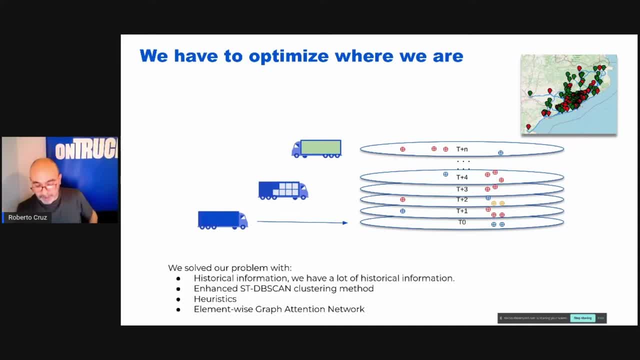 because the graph attention network allows us to represent the power of the graph topology and propagate all the node information to the edge via an attention mechanism, And this allows us to learn which is the best route in this moment to produce the less emission with the vehicles that we have and the order that we have. 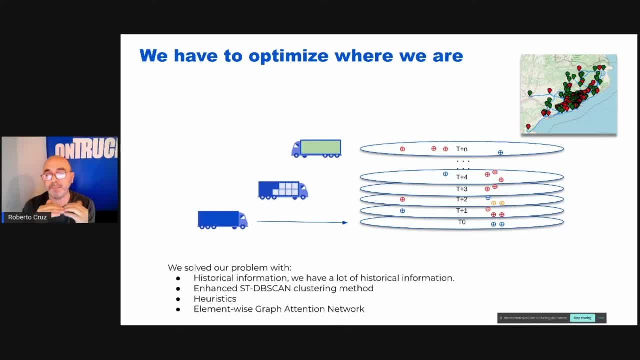 We have to consider that most of our market is a spot market. This means we don't have vehicles. we don't have our own fleet. We have to use fleets that are available every time and in every location. This means that not all the vehicles are available. 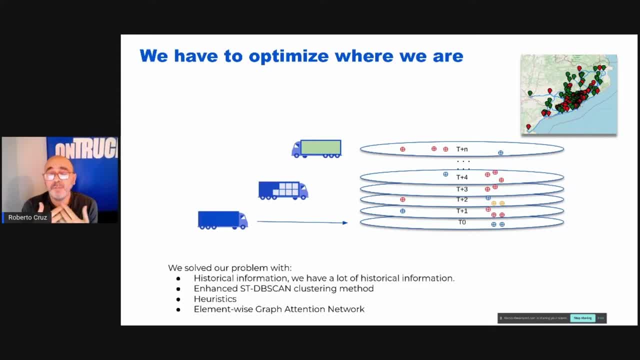 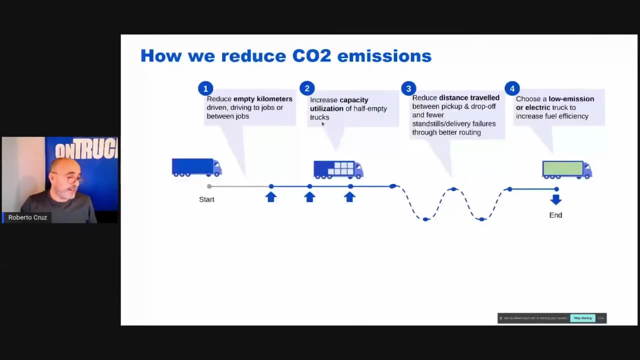 only some of them that we can use and we have to maximize their utilization, reducing the distance And we reduce emission. Finally, how Well in regional LTL or in national and international LTL? LTL is less than 3%. 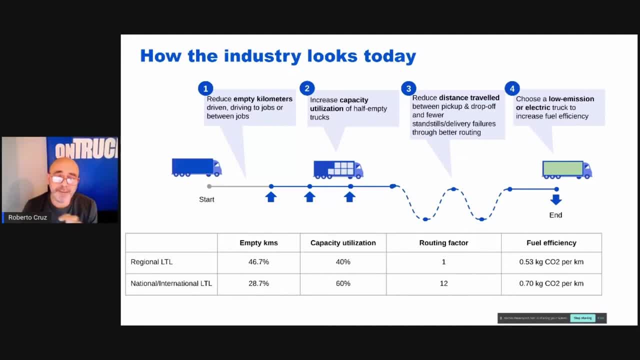 This means that we are collecting different loads and fulfill a track. In the past, we used to have 46% of the vehicle empty and we used to drive with empty 46% of the distance and use the vehicle up to 40%. 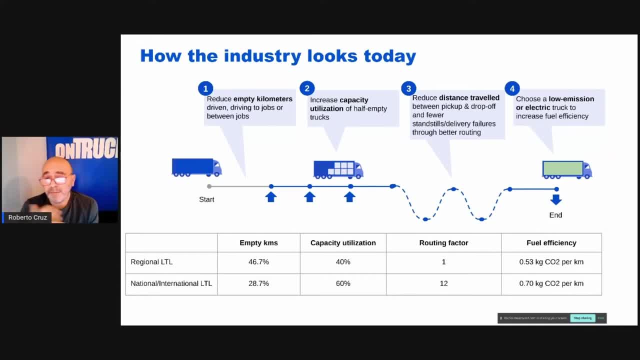 So this means that we are collecting different loads and fulfill a track And we are not very efficient. then with the full emission, We are emitting a lot of CO2. And in national and international we are able to drive less anti-kilometer. 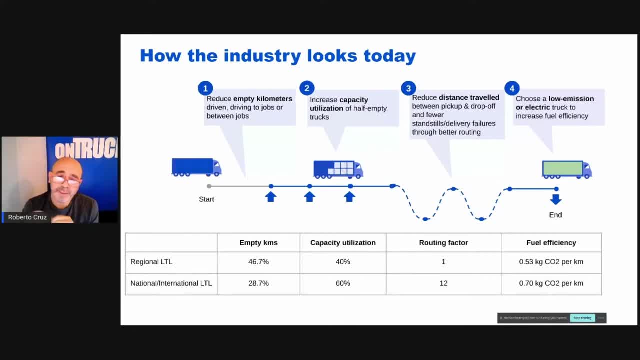 because the distance is bigger, have a bigger utilization of the vehicle and because we are able to have a better routing factor. With our new algorithm, we were able to reduce the anti-kilometer in regional LTL from 46% to 20%. 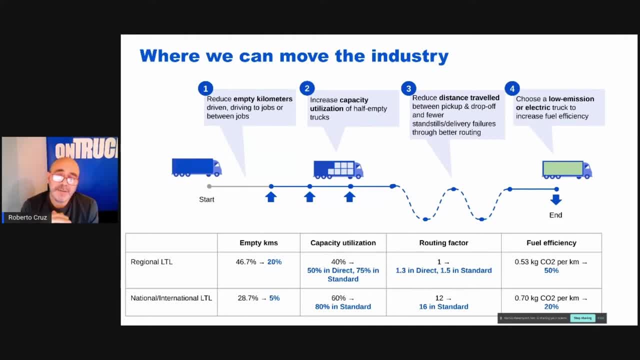 We were able to increase the utilization to 50% in direct. This means that pure spot market increased 10% the utilization of the vehicle and 75% in the whole marketplace in the all day program And this provides to us that, finally, that we reduce the emission to the atmosphere. 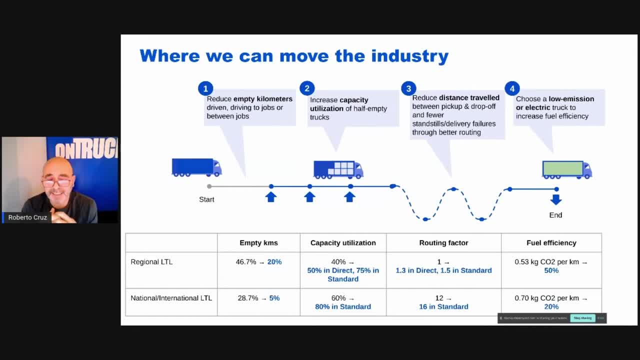 in 50% in regional LTL. That is a lot In national and international LTL. we reduced the anti-kilometer to 5%, We increased the utilization to 80% And this has an impact again of another 20% on the emission to the atmosphere. 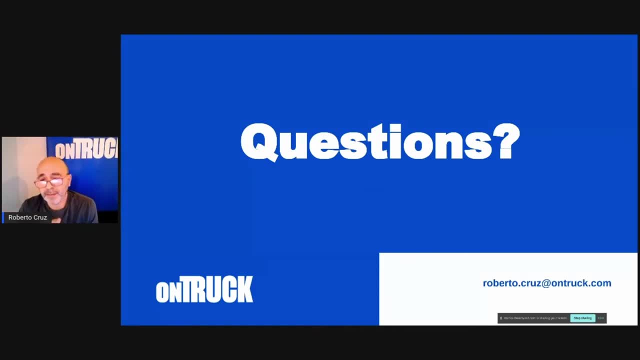 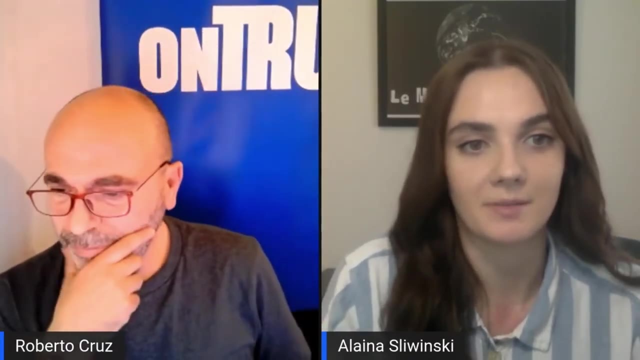 That's all. You can contact me here for any questions or through my email. Any questions are welcome. Thank you, Roberto. That was a great presentation And, as I already mentioned, a topic that a lot of people are curious about and want to improve upon. 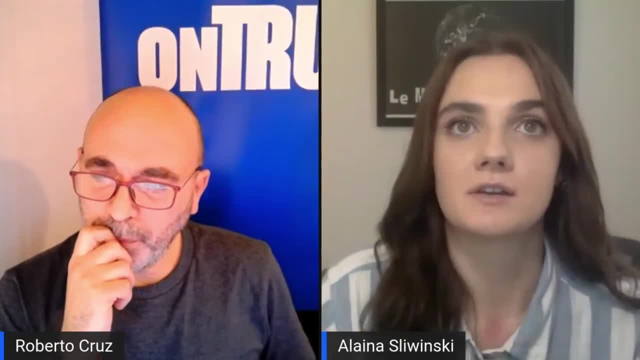 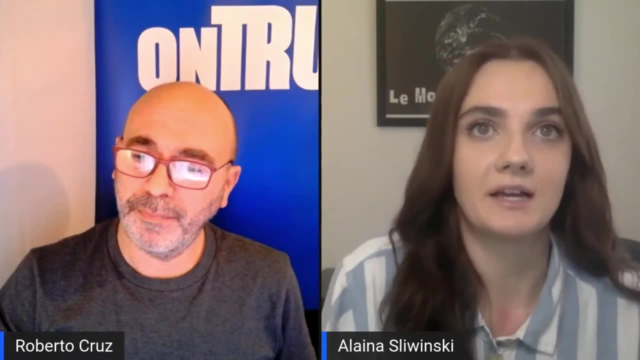 So we do have time for a couple of questions. I think you already covered the impact of reducing the CO2 emissions, But we're curious to know: is there a stage of the supply chain associated with having the highest CO2 emissions? Sorry, 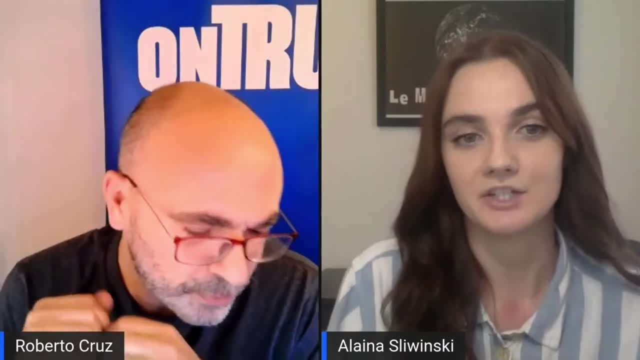 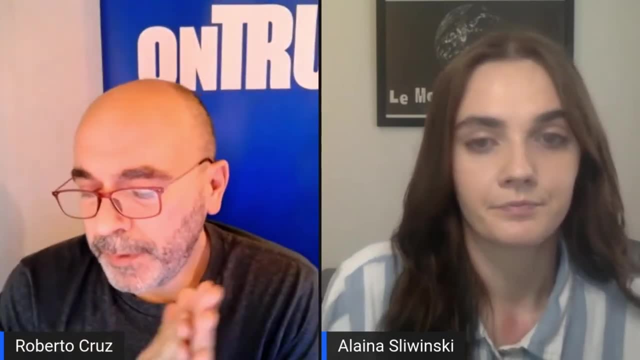 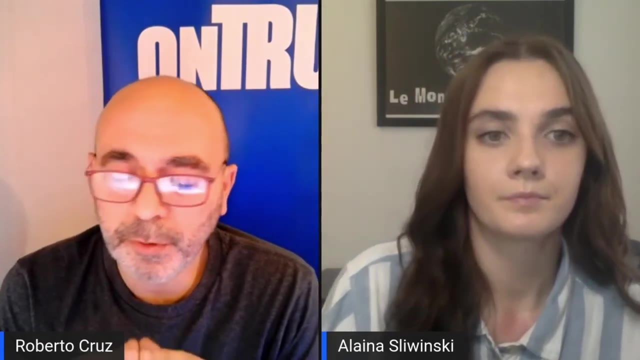 Is there a particular stage within the supply chain process that is associated with having the highest emissions? Yeah, It's normal. In logistics the highest emissions comes because it's difficult to optimize the vehicle utilization because normally you cannot do it in real time. 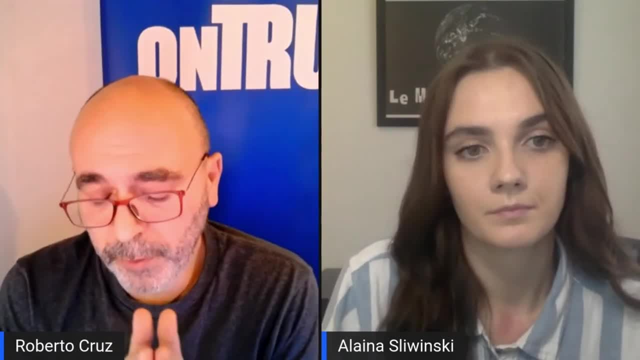 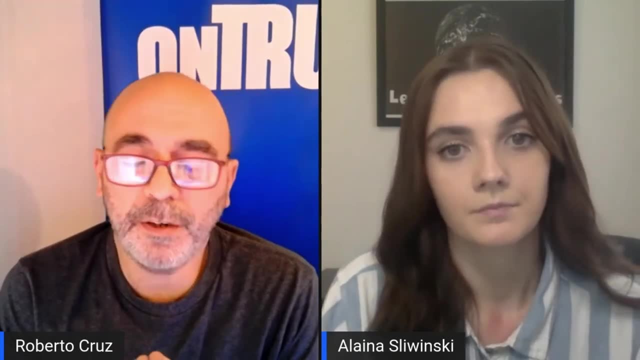 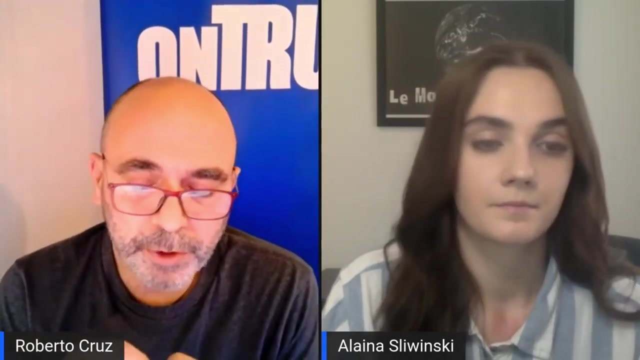 The problem of routine optimization is an NP, non-polygonomial optimization. It's a time problem. That means that needs a lot of capacity of calculus to solve the problem. This means that today we are not able to solve closing to real time. 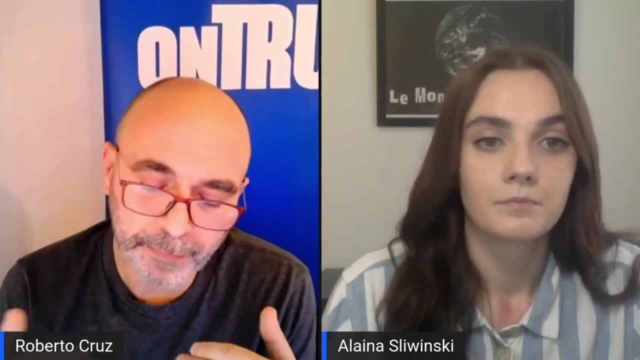 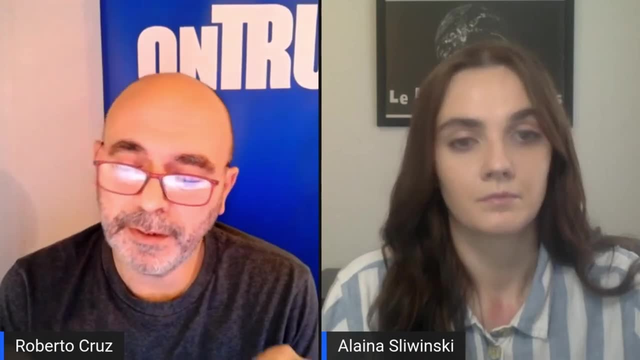 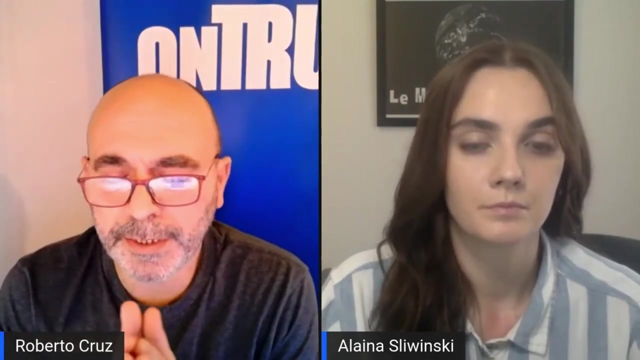 What we found is a way that, with historical data and all the cluster information, to reduce the depth of the calculation and have the result close to real time. This means that our average calculation time is less than that. It's less than 300 milliseconds for big problem. 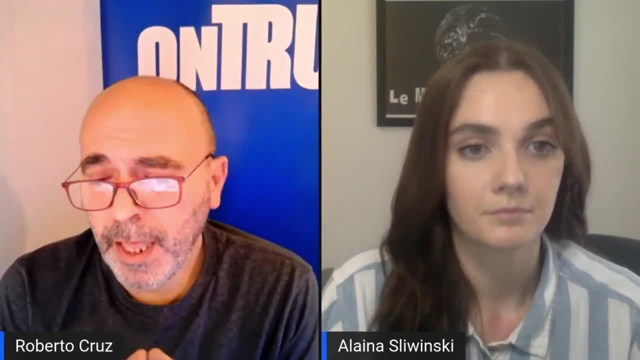 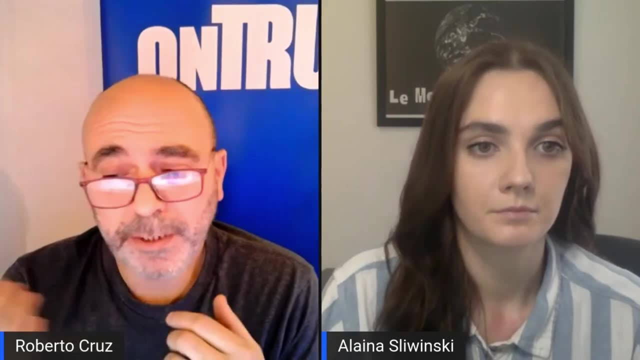 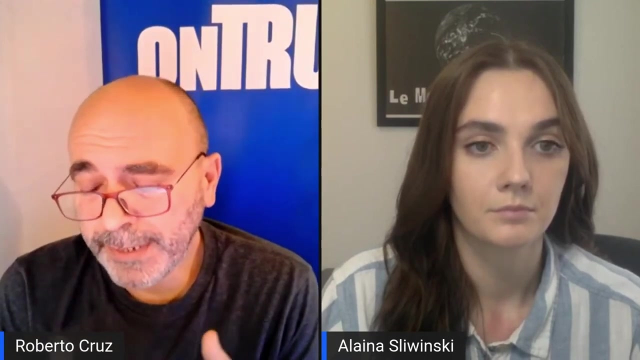 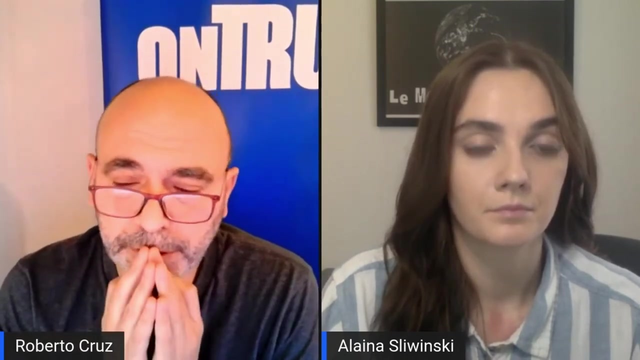 I say 100 points problem and less than two minutes for 500 point problem with close to the best solution, with 95% closest to the best solution. That is big enough for our market and improve a lot the emission, the reduction in the emission that we produce to the atmosphere. 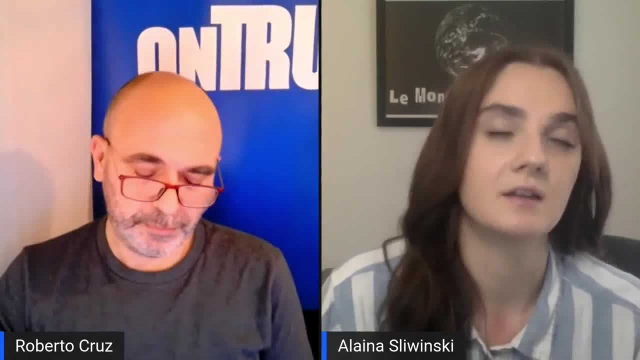 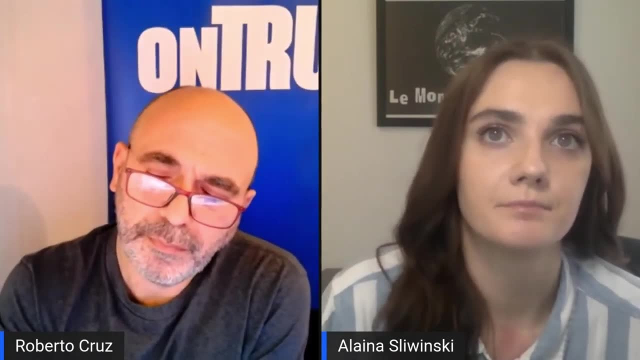 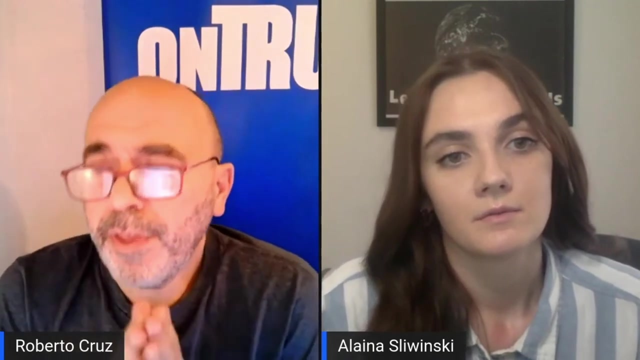 Absolutely. Then, with that being said, from your analysis, what's one of the most feasible or easiest ways to massively adopt methods for reducing CO2 emissions? and logistics, What's something that everyone can easily start with. I think the first thing is just to understand. 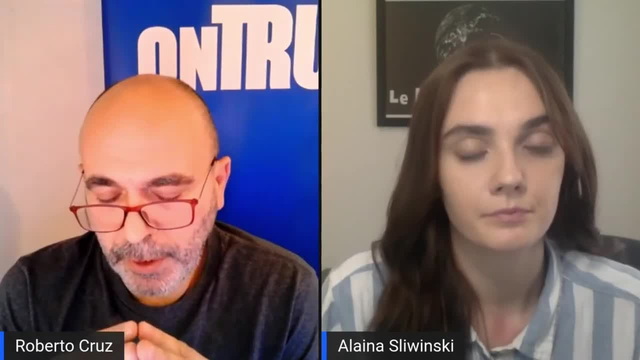 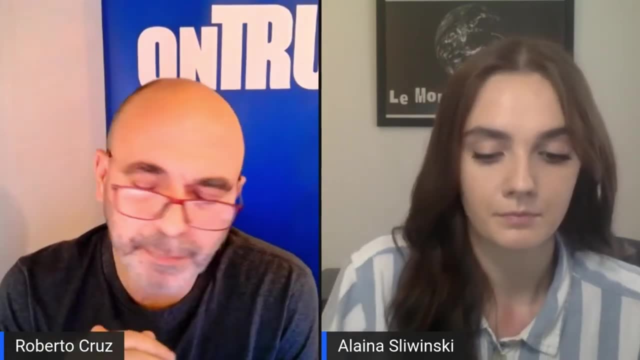 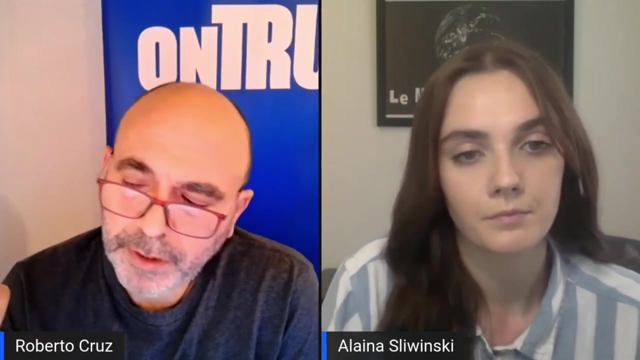 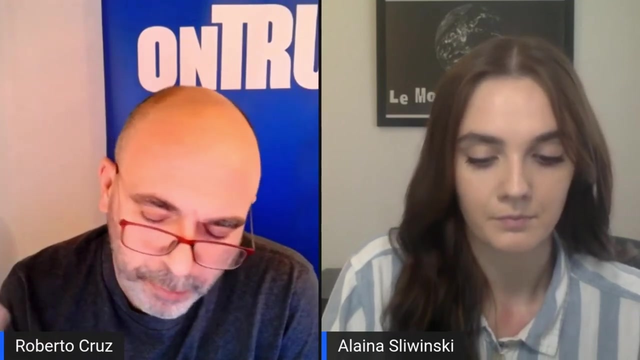 how you can use the basic algorithm to reduce the anti-kilometer. The anti-kilometer is the big problem that we have in the industry: Anti-kilometers and anti-tracks. It goes to the government center, European community information, But we've discovered that 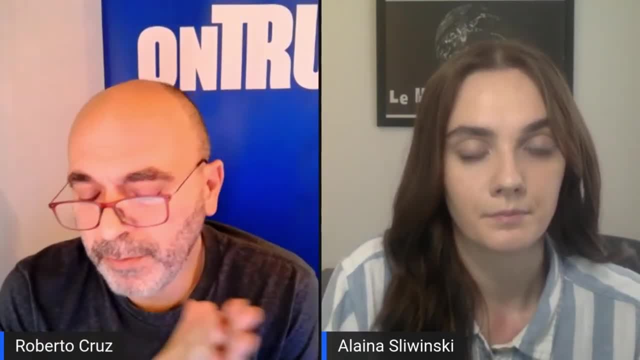 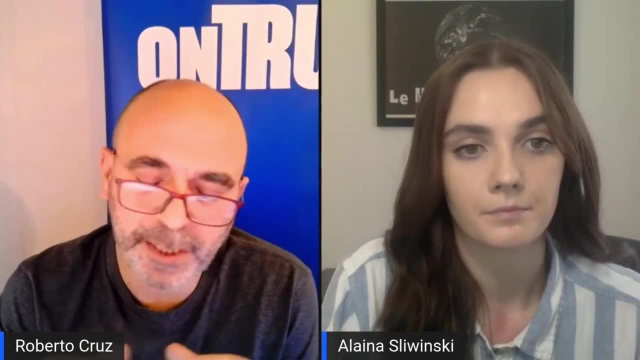 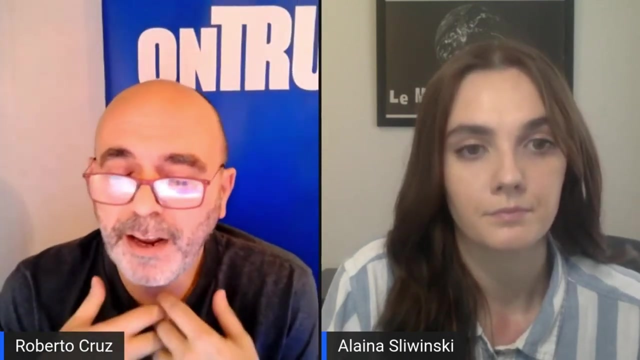 as average in Europe. we have over 50% of our track that are now traveling across Europe are empty. That is a lot because it's emission for moving nothing- moving air- And if we can reduce just those emissions just using more the vehicles. and reduce the kilometers. just with optimization of the problem, it will be good for the planet. Awesome Thanks for sharing that one. To follow on, will these changes to supply chain be hard to maintain or is the harder part in initiating these kind of methods for reduction? 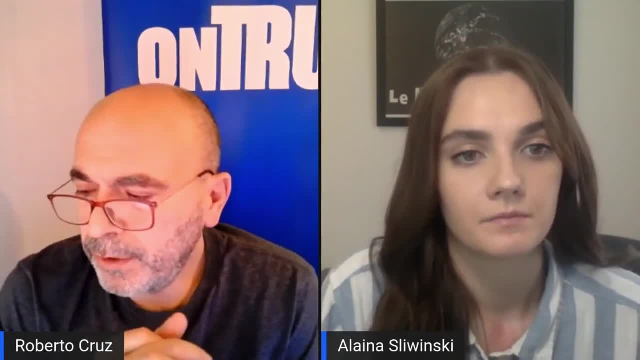 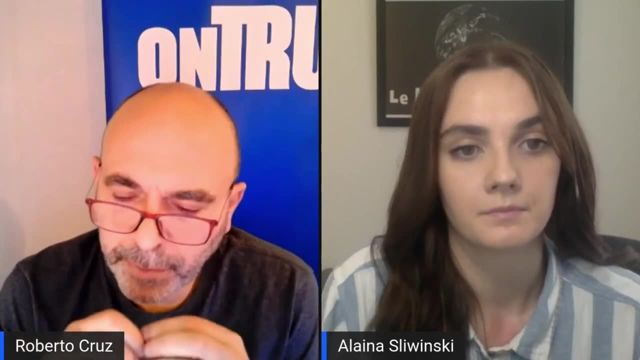 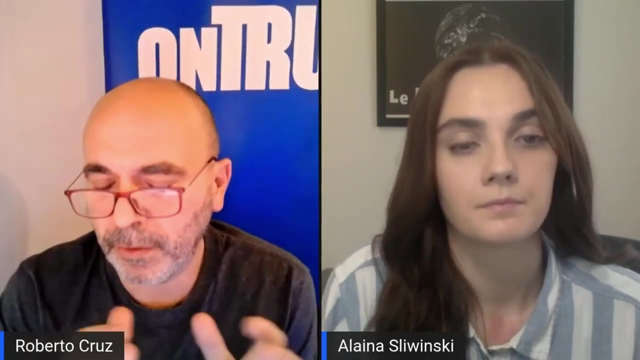 I think it's initiating more and more customers asking to have the report We are providing to them right now: report on the CO2 emission, just per order. It means that they know how much they will emit with their order And, finally, what really we emit with their order. 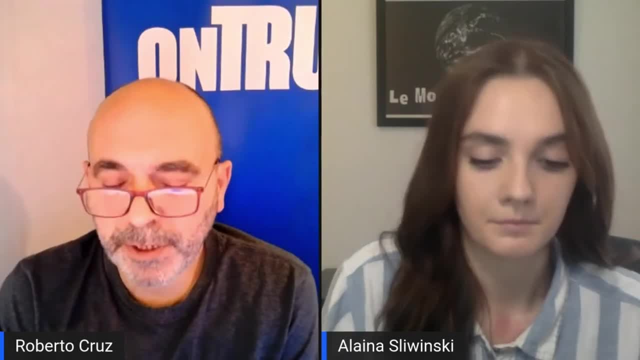 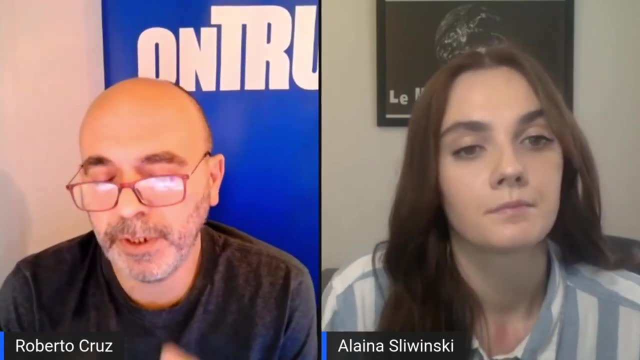 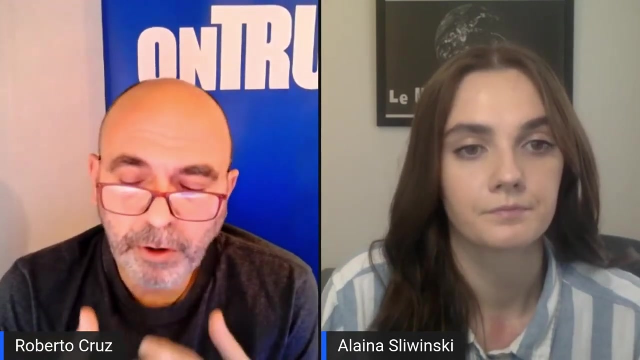 in order to have a clear conscience about the emission that any merchant that we move, the impact of any merchant that we move in our planet, Companies like L'Oréal right now forced to have this information in all the report, in all the billing. 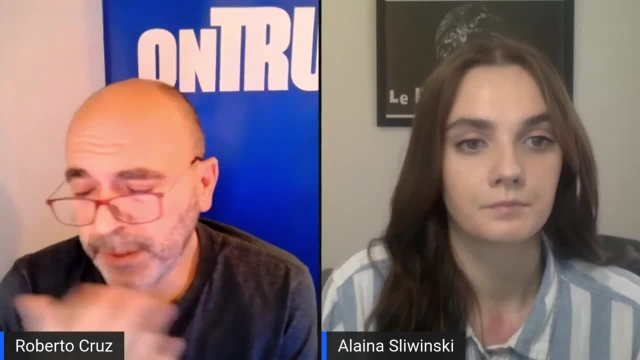 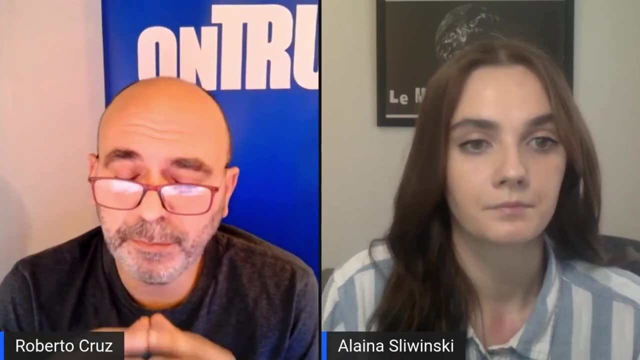 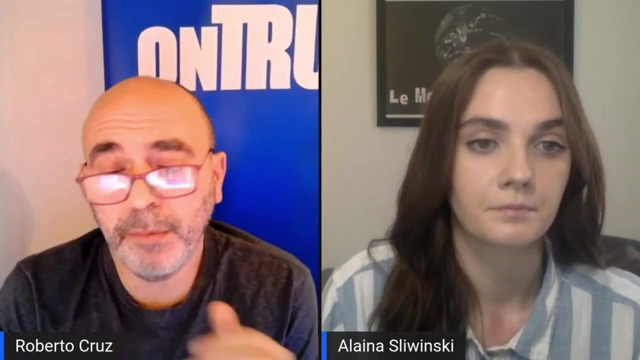 because it's important for them. And recently, companies like Amazon, like IKEA and other ones just say that to 2030, 2030, they will be emission free or emission compensate in all the movement of merchants. That's a bold target.